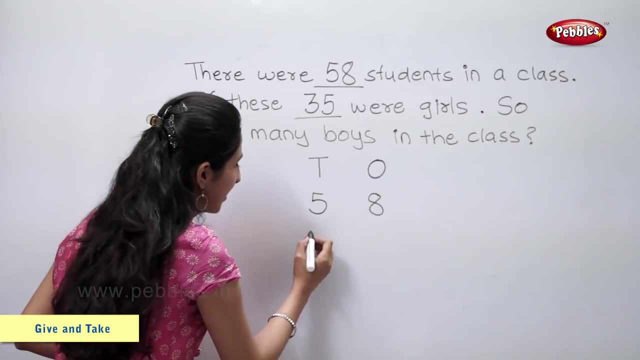 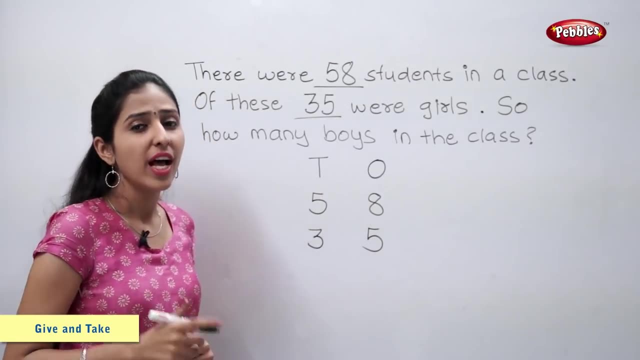 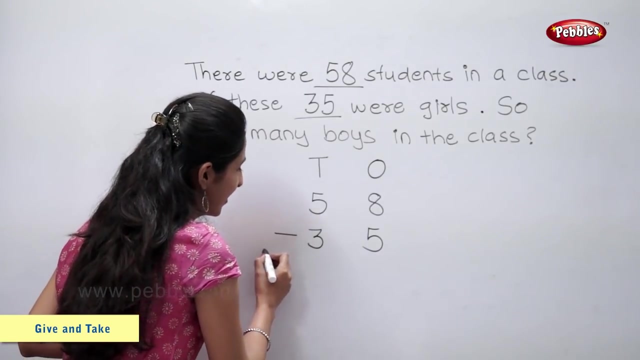 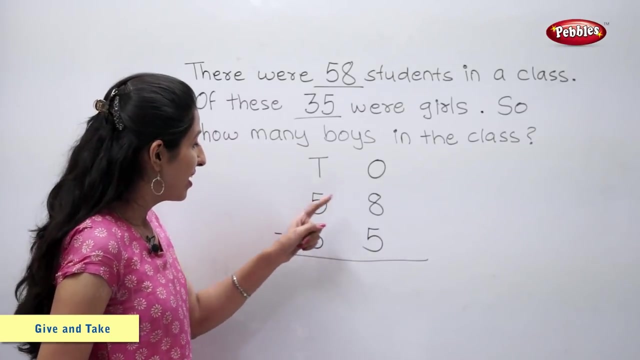 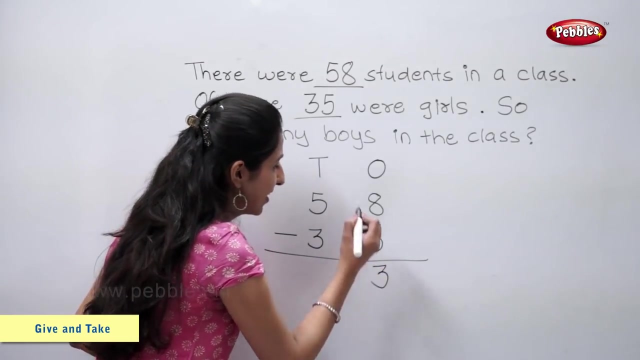 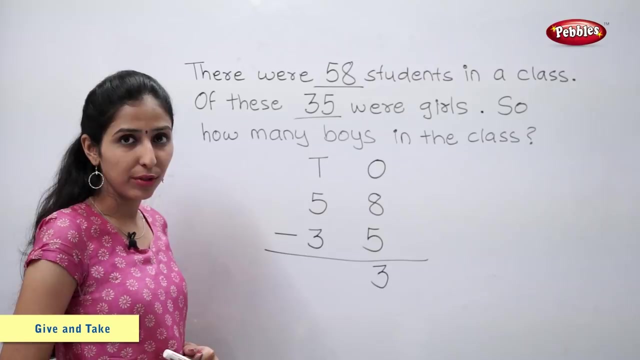 3 tens 5 ones. 3 tens 5 ones. Now, as we have to find number of boys, we will subtract. Let us subtract ones first: 8 minus 5 is equal to 3.. Now, tens 5 minus 3 is equal to 2.. 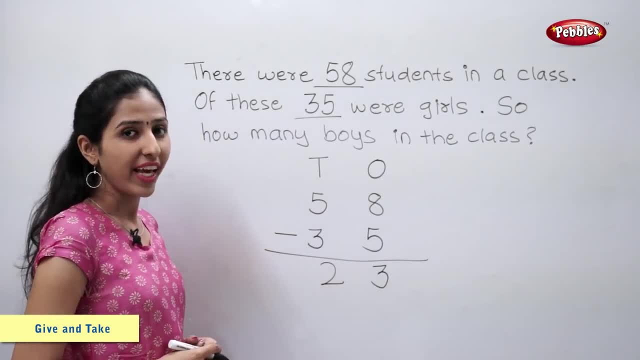 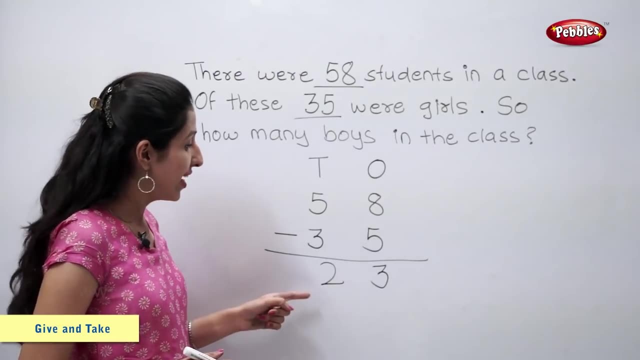 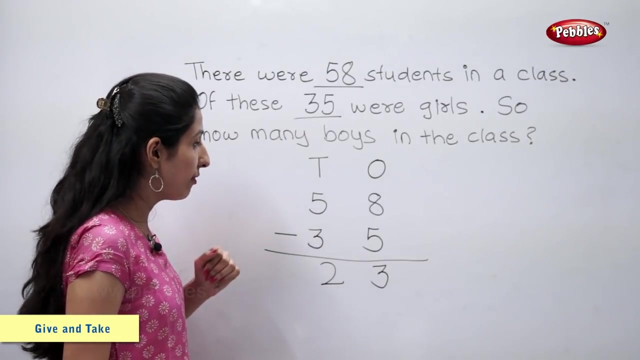 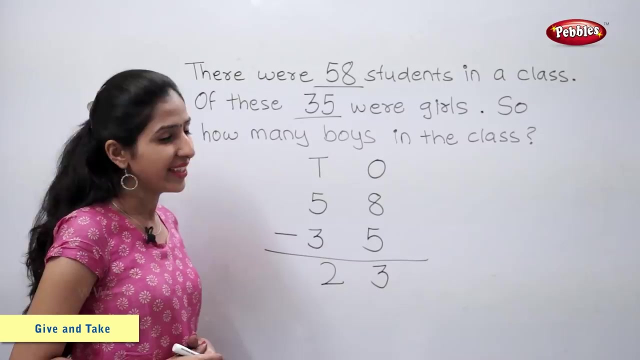 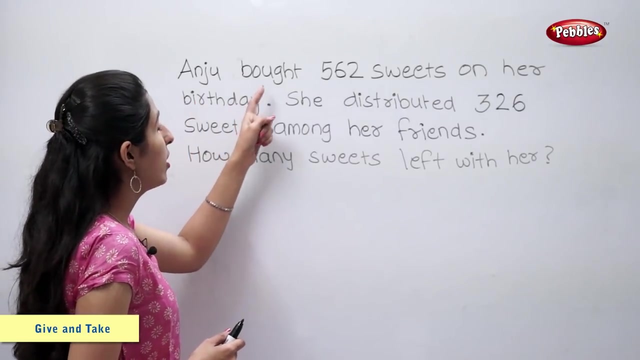 So now we have 2 tens, 3 ones. That is number 23.. So 58 minus 35 is equal to 23.. So 58 minus 35 is equal to 23. 23. So there were 23 boys in the class. Now let us look at this example: Anju bought 562 sweets. 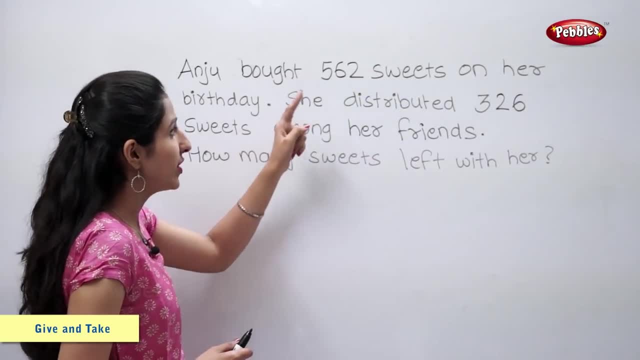 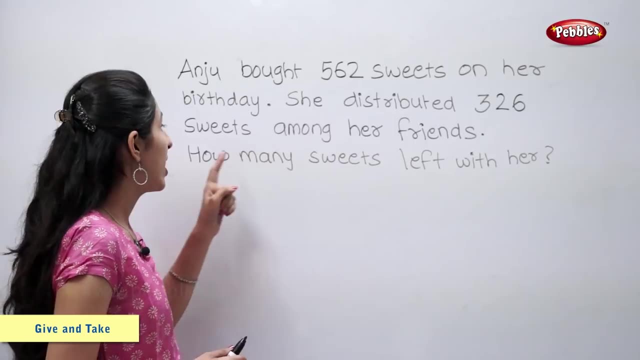 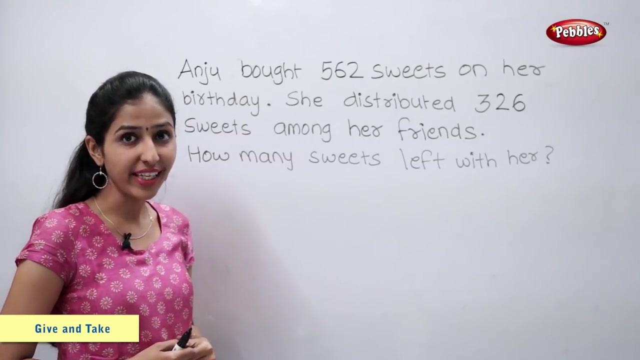 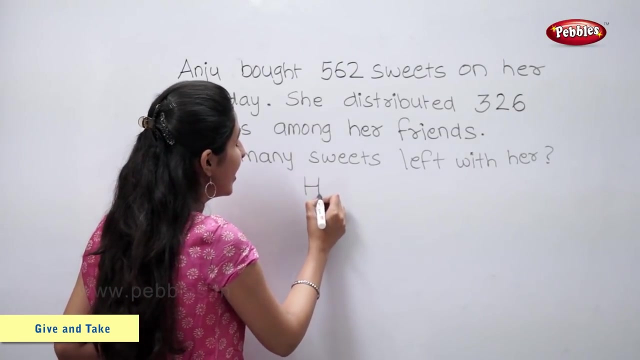 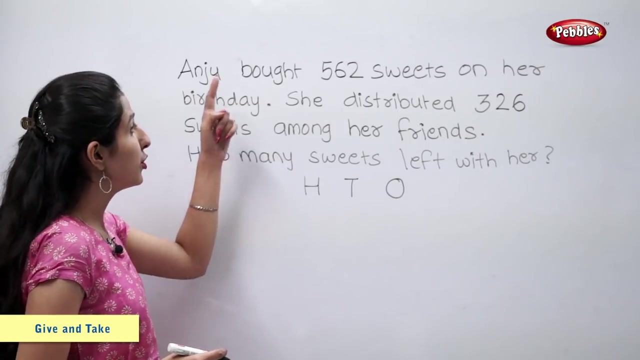 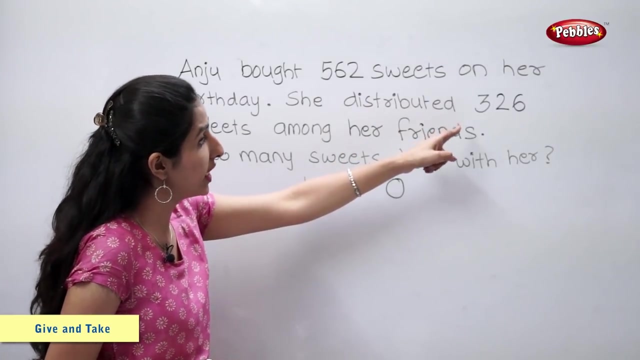 on her birthday, She distributed 326 sweets among her friends. How many sweets left with her Students? let's solve this sum using hundreds, tens and ones. So let's write hundreds, tens and ones. Anju bought 562 sweets. She distributed 326 sweets. Now we have to find. 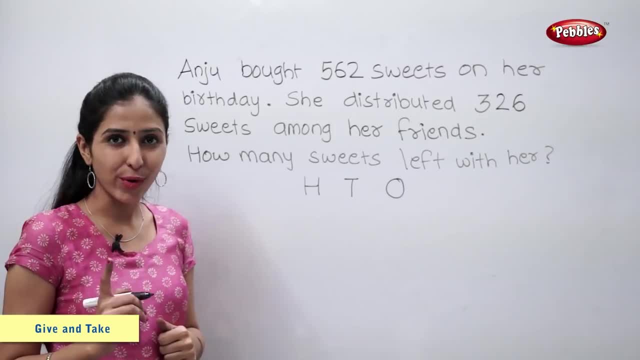 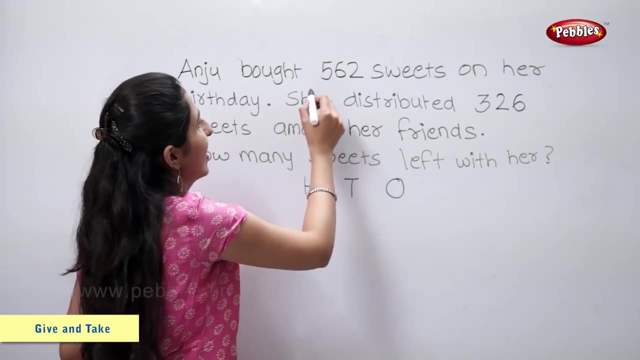 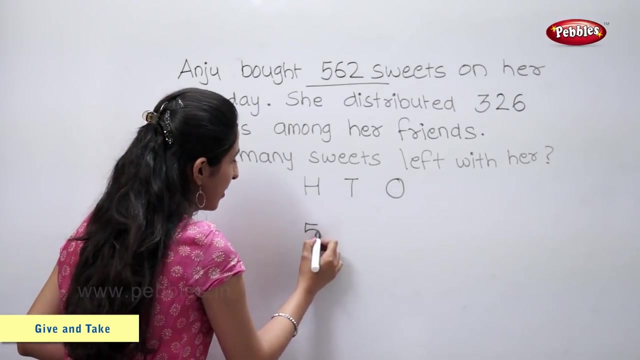 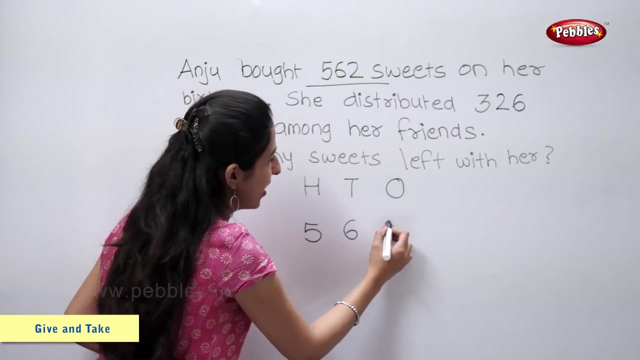 362 sweets Now. we have to find 362 sweets Now. we have to find 362 sweets Now. we have to number of sweets left with Anju. So we will subtract 562 sweets. 562 means 5 hundreds, 6 tens and 2 ones. 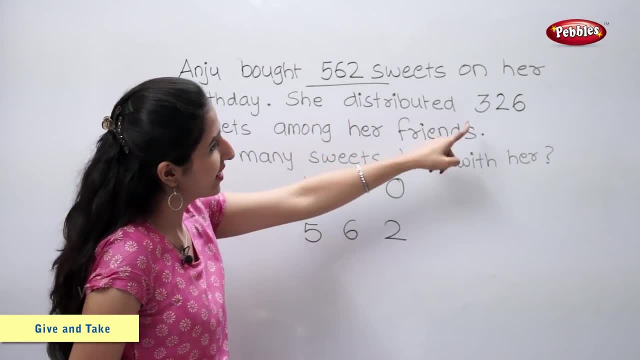 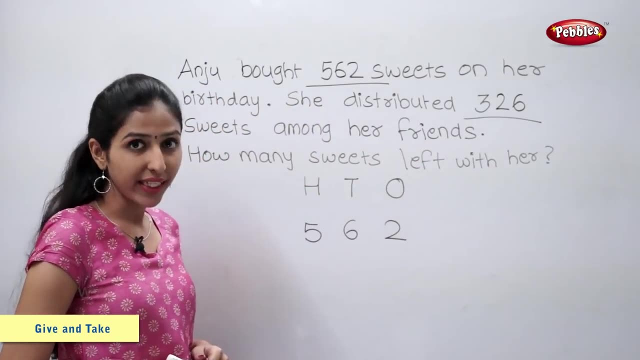 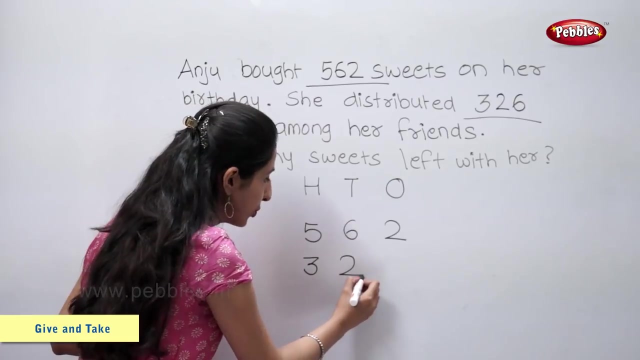 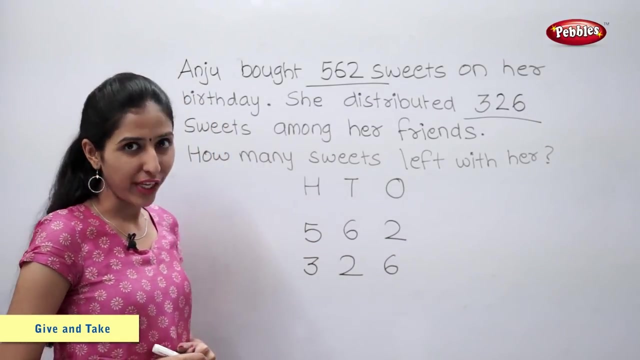 Students. let's solve this sum using hundreds, tens and ones. She distributed 326 sweets. Now we have to find 362 sweets. Now we have to find 362 sweets. Now we have to count it: 326 means 3 hundreds, 2 tens and 6 ones. We have to find number of sweets left with Anju. 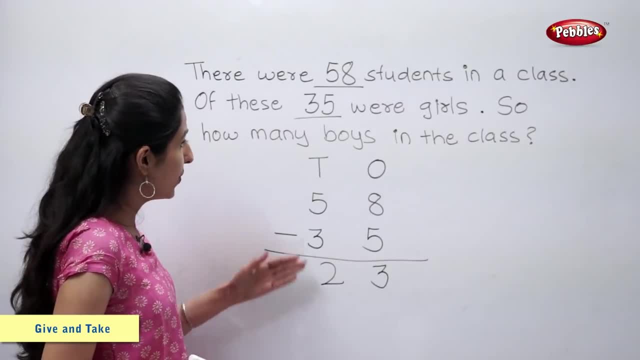 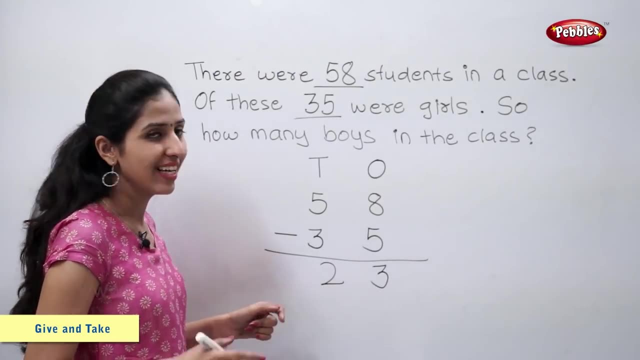 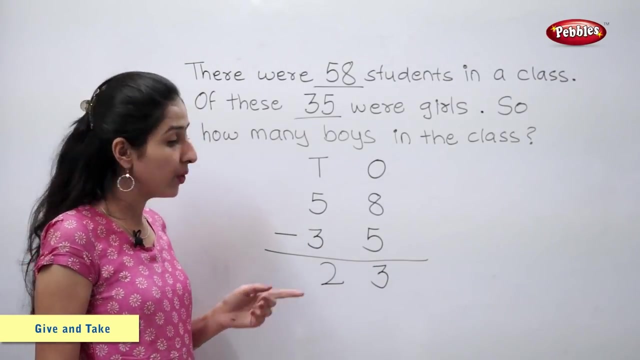 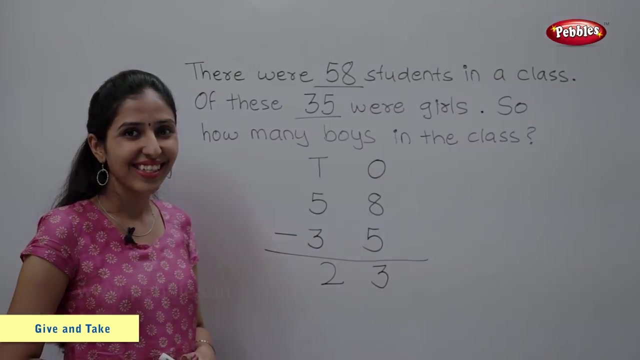 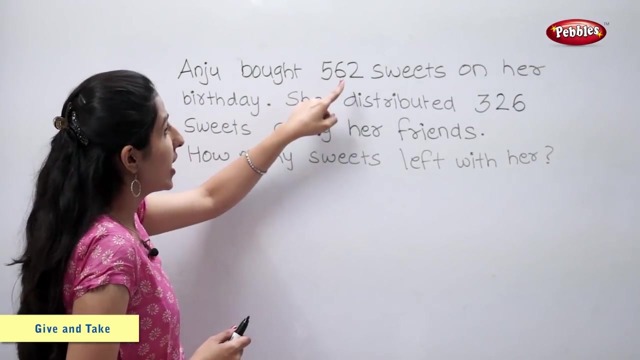 So now we have 2 tens, 3 ones, That is number 23.. So 58 minus 35 is equal to 23.. So there were 23 boys in the class. Now let us look at this example: Anju bought 562 sweets on her birthday. 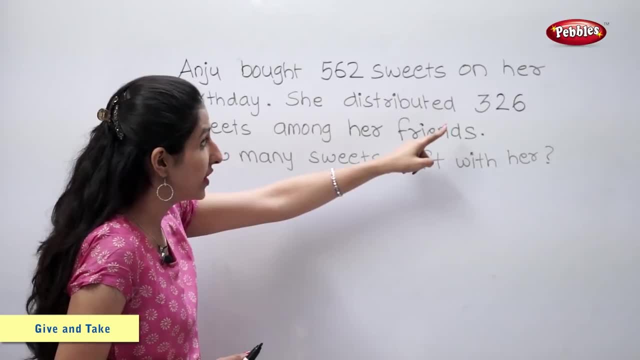 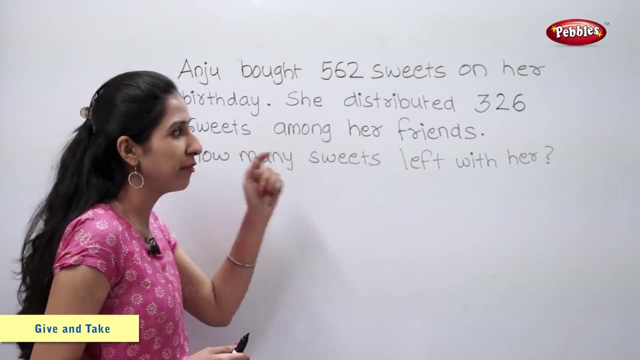 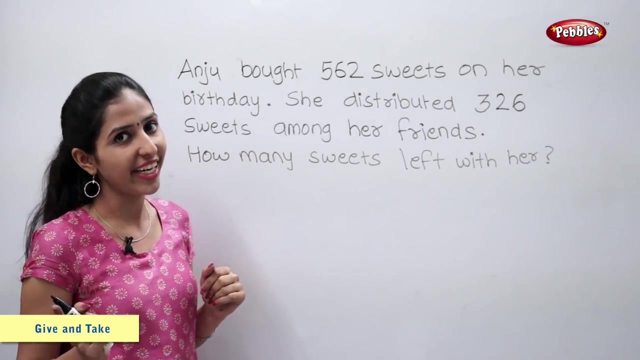 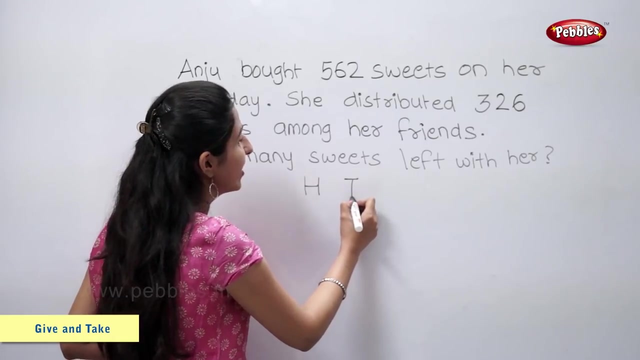 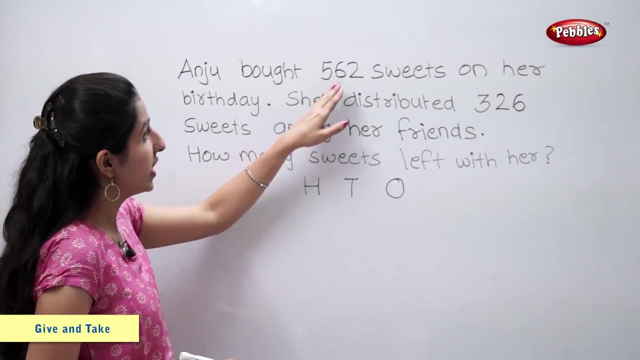 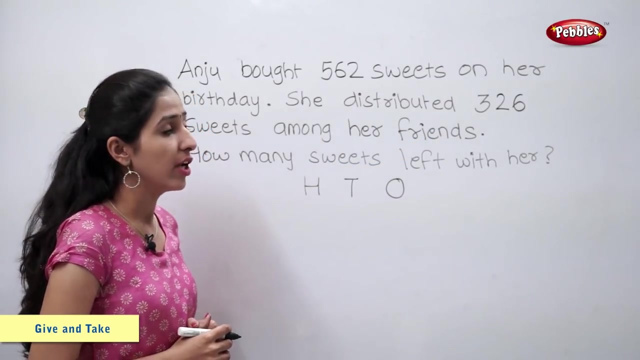 She distributed 326 sweets among her friends. How many sweets left with her Students? let's solve this sum using hundreds, tens and ones. So let's write hundreds, tens and ones. Anju bought 562 sweets. She distributed 326 sweets. Now we have to find. 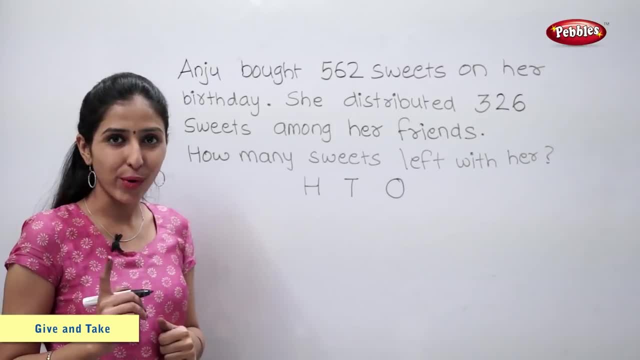 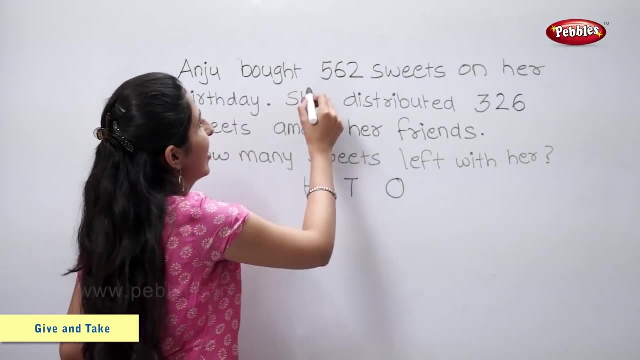 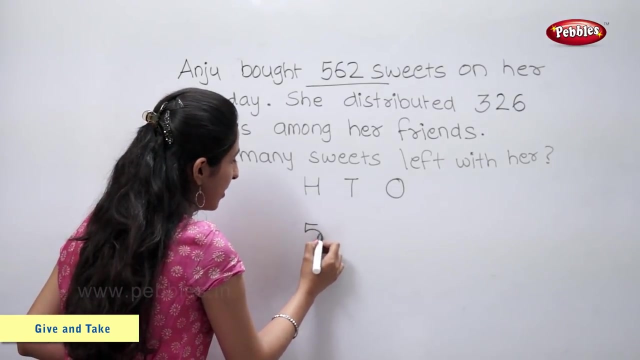 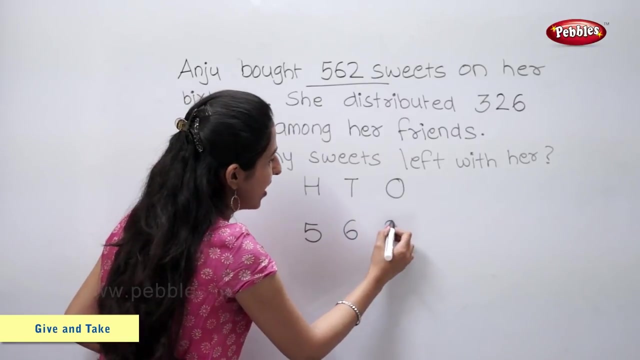 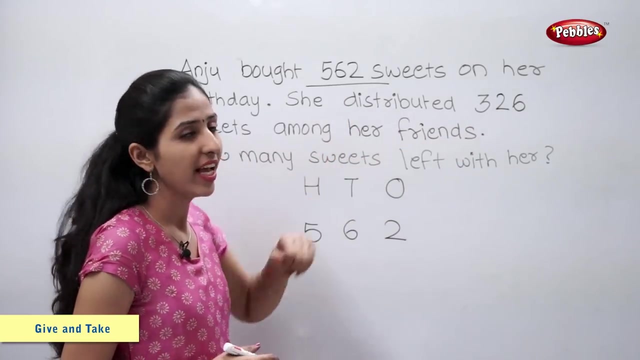 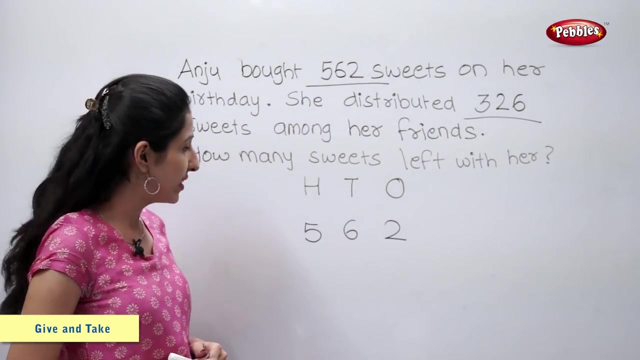 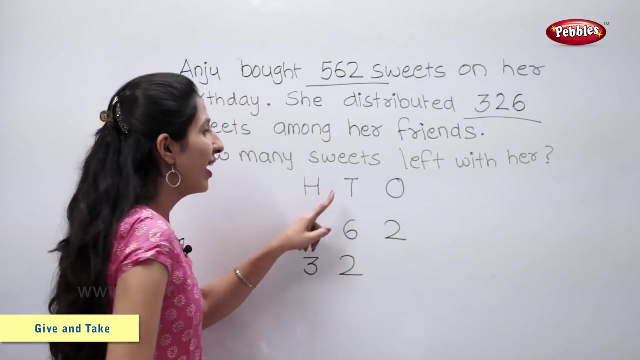 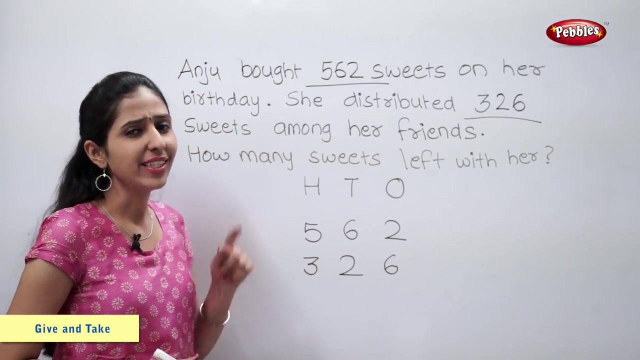 362 sweets, Number of sweets left with Anju. So we will subtract 562 sweets. 562 means 5 hundreds, 6 tens and 2 ones. She distributed 326 sweets. 326 means 3 hundreds, 2 tens and 6 ones. We have to find number of sweets left with Anju. 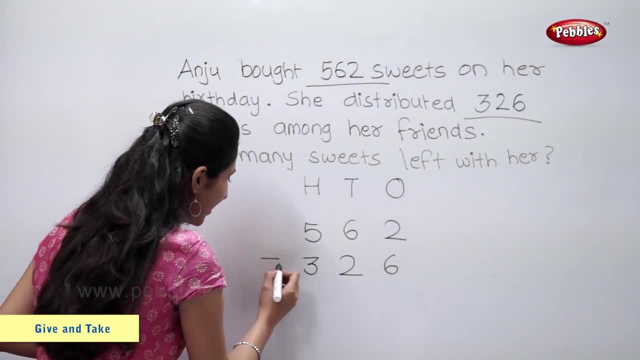 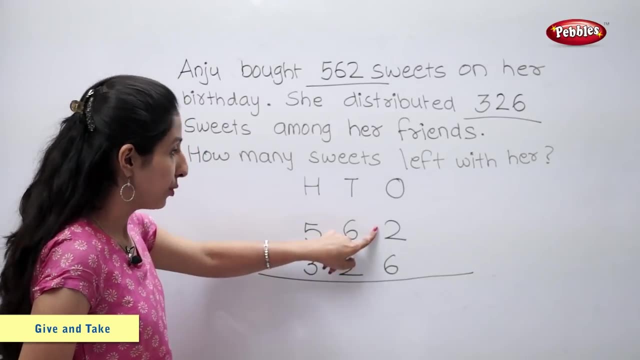 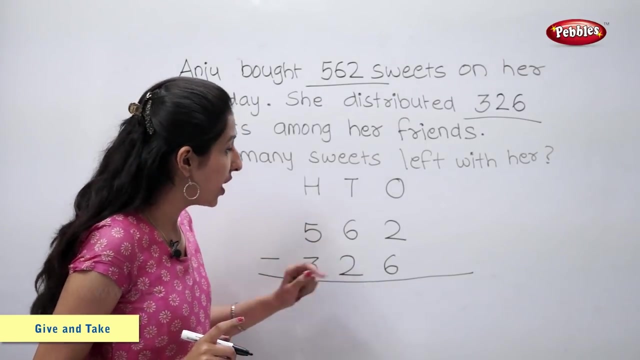 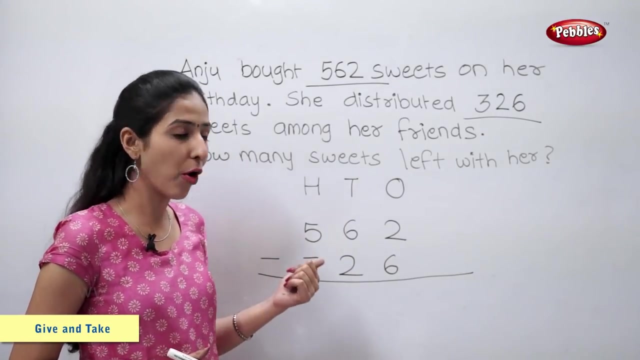 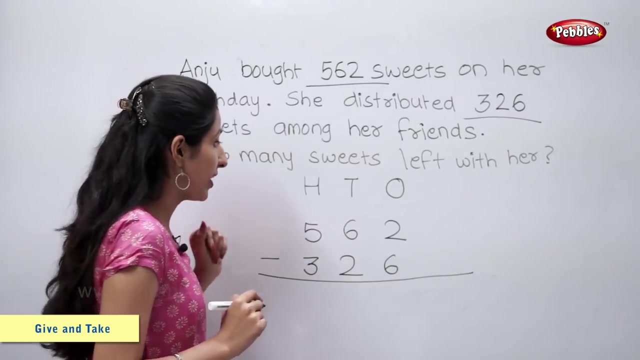 So let's subtract. Let us subtract ones first: 2 minus 6 Students. we cannot subtract 6 ones from 2 ones, So we will borrow 1 tens from tens column. 6 tens minus 1 tens is equal to 1 tens from 1 tens column. 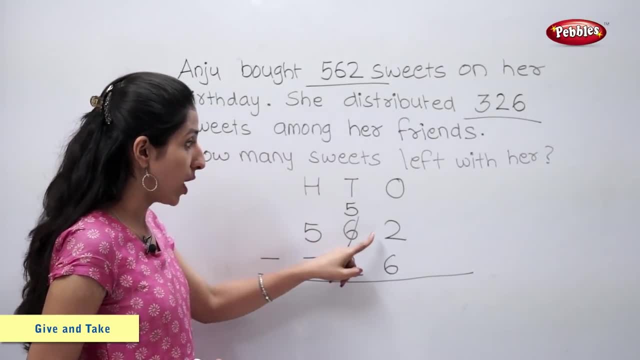